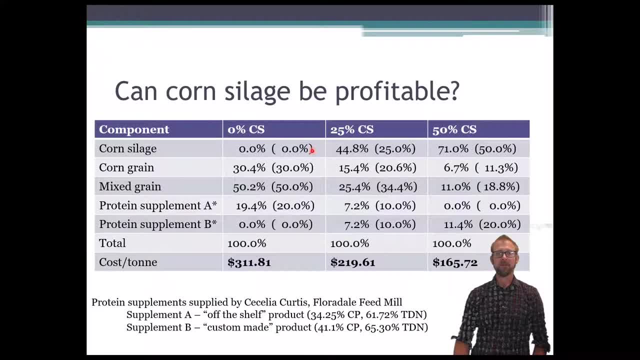 more people. So what we did is we fed either no corn silage at all, 25% corn silage on a dry matter basis, or 50% corn silage on a dry matter basis, and the ingredients we substitute for that would have been corn and mixed grain, which of course is oats and barley. We used an off-the-shelf 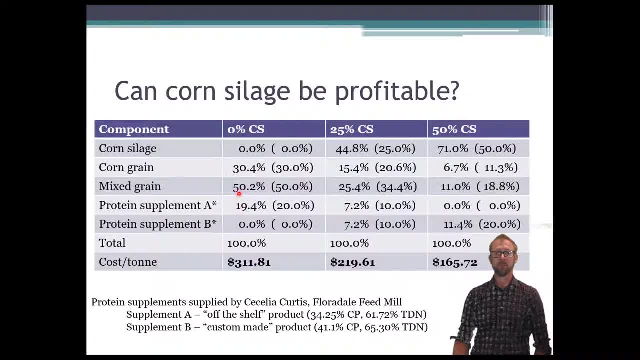 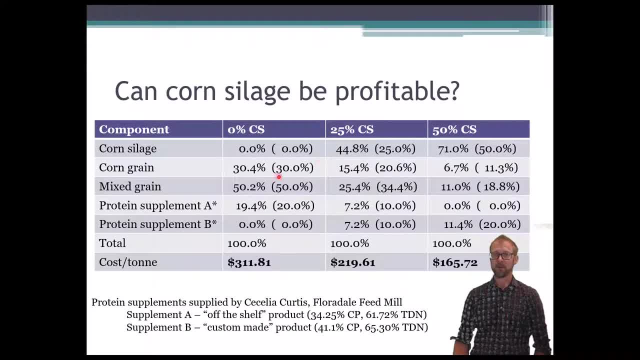 in the 25% corn silage treatment would have been a half the protein supplement from this from the 0% and half from the 50%. And as you can see right at the top, just looking at the cost per ton of these feeds, the cost for the corn silage treatment was considerably cheaper than than feeding a full 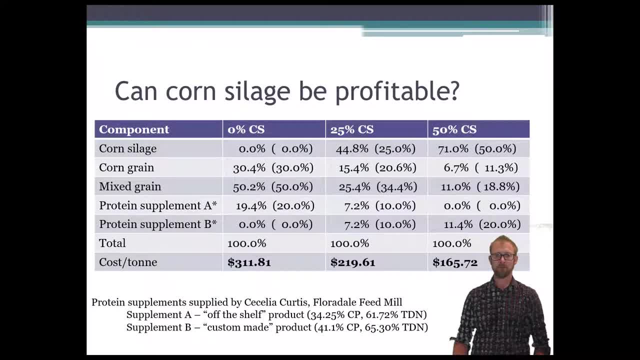 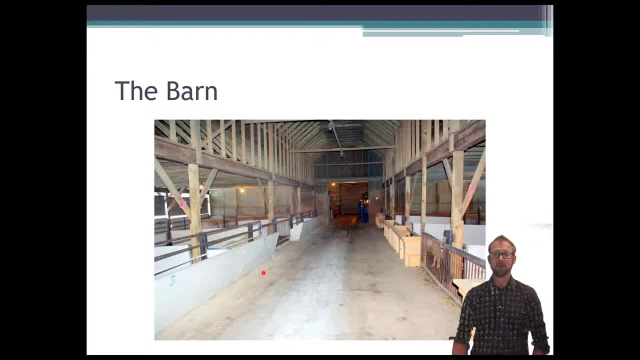 grain diet and these prices were prices at the time of when the trial occurred. This is a bar that we did. the project in The project was: this was one of the early projects we did, so we had half cement bunks, half were wood bunks at that time and the pens were about 16 foot wide and about 20 foot. 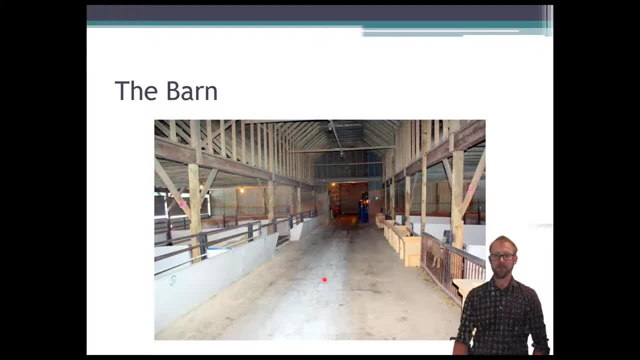 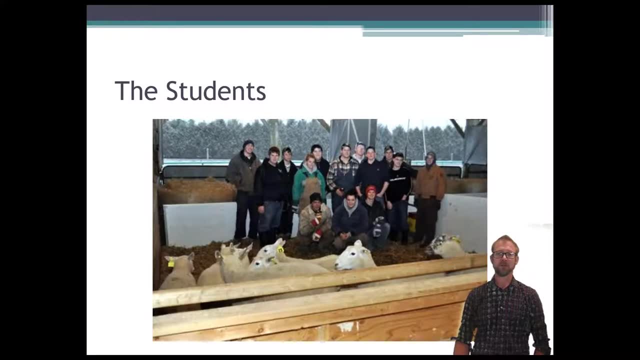 long and we had enough bunk space for all the lambs to be able to feed at the same time. I try as much as possible to get students involved in our project, so this is a group of students that were involved in that one, and I think it's good for their learning. they get to see different things, how. 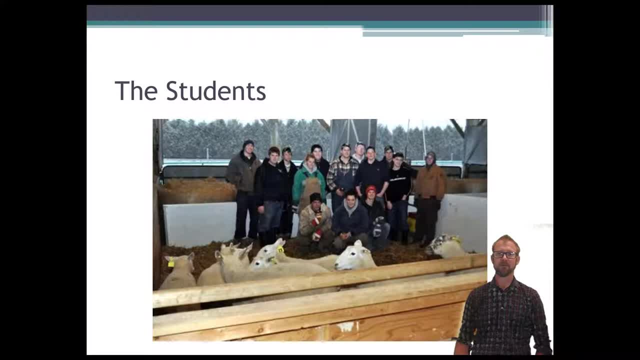 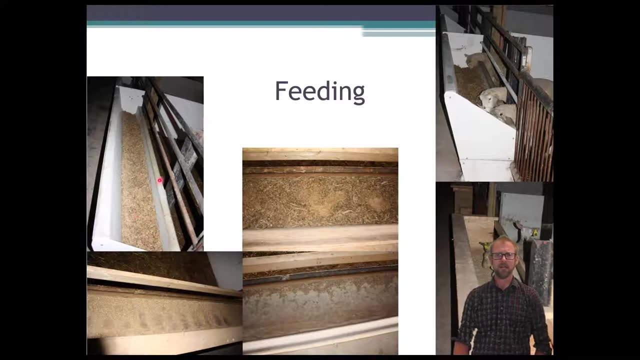 and get to measure feed intakes and so forth very closely, watch the animals very closely and- and of course it also helps with all the labor of doing a project like this- Here you can see the feeding that we did right here you'd see the height the grain when it was first put in. this would be the 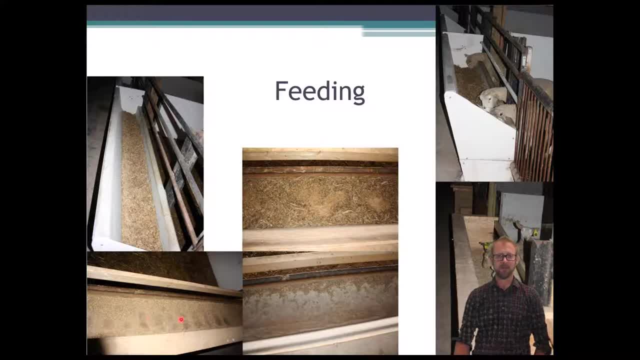 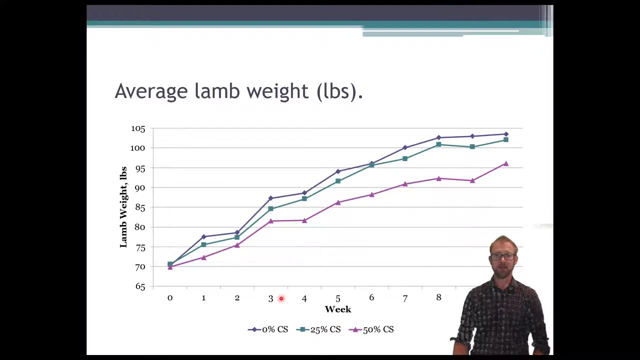 corn silage when it was first put in and you can see after time the grain was eaten down to this level and the corn silage treatment would be eaten down to that level. We tried to feed for a 5% refusal every day. If we look at the lamb weights over the different weeks that the trial went on, you can see that the 0% and the 25% corn silage 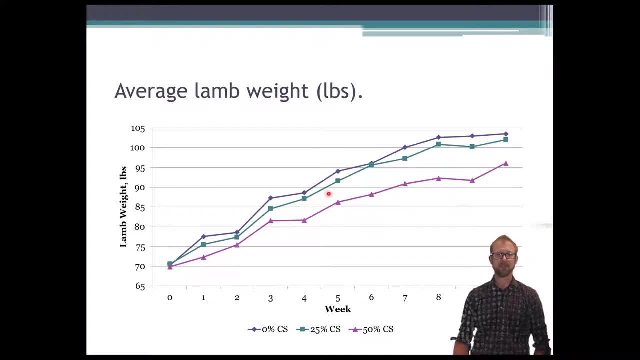 treatments they grew, basically the same rate. the 25% might have been slightly lower but all in all they they tended to keep fairly well up with the lambs going all the way through that were on the high grain diet, whereas you can see that the ones on the 50% corn silage, especially by about week. 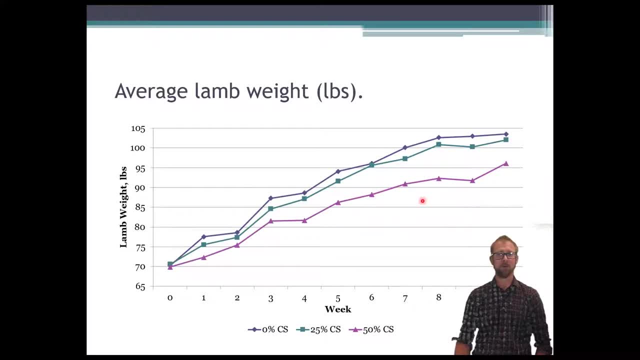 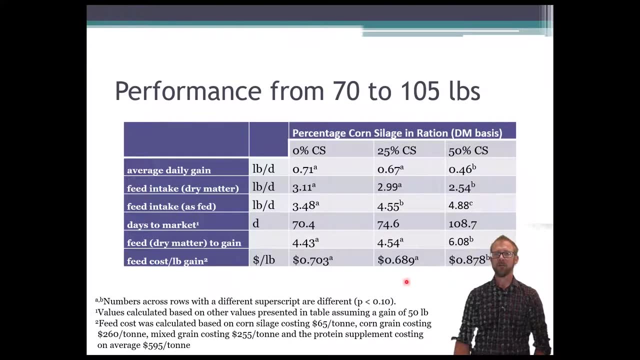 three, four. they really kind of fell off and were unable to keep up their growth rates, as they as was able to happen with the higher grain diets. If we look at that in table form, they would. their lambs were about 70% before we could start collecting the data, and that's just because from the time we get them in. at that time we were still buying them from sale barn- we had someone helping us with that- and by the time you get them in, get them transitioned and ready to go, that they were a little bit heavier- I'd like to start at about 60 pounds- and they land up, going on average at 105. pounds. I would have again like that, keep them for an extra week, but that was just how it worked out for being able to get them into the meat lab to get the analysis done in them in there as well. When we look at the average daily gain over this time, though you can. 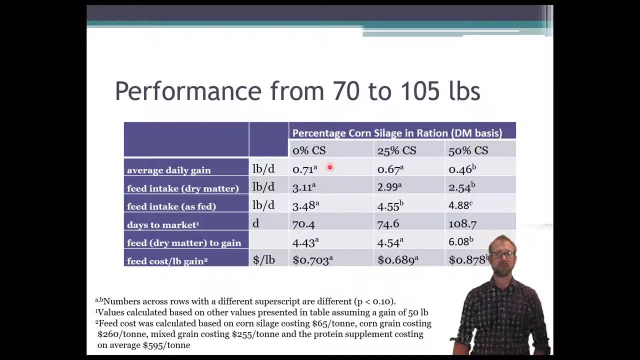 see, yeah, they grew. the 0% corn silage grew at about 0.71 pounds per day, and then the ones on the 25% corn silage. very similar. when you see two letters like that, the little subscript AA across the treatments, like that, that it tells you that those two are not significantly different, whereas 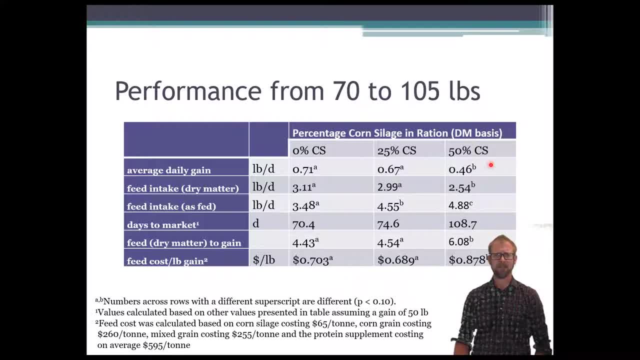 this one here is a B. it was significantly different from the other two in this case and exactly the the 50% corn silage lambs grew slower. they were unable to keep up, and we saw that on the previous table as well. if we look at the feed intake across the whole trial for 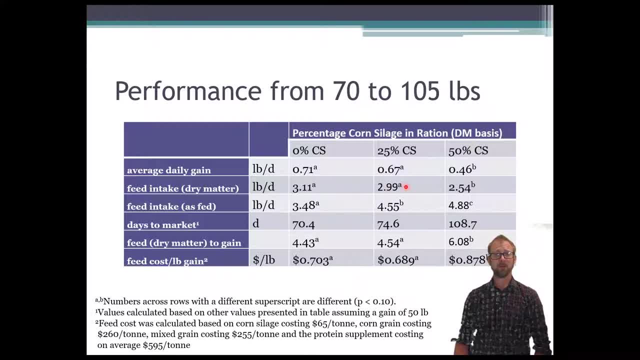 these ones, these guys. it consumed about 3.1 pounds, about 2.99 pounds again. there was not a significant difference between those two treatments. however, the feed intake for the 50% corn silage ones was significantly lower feed intake, the feed intake on an as-fed basis, this probably. I mean it should make sense the more corn silage 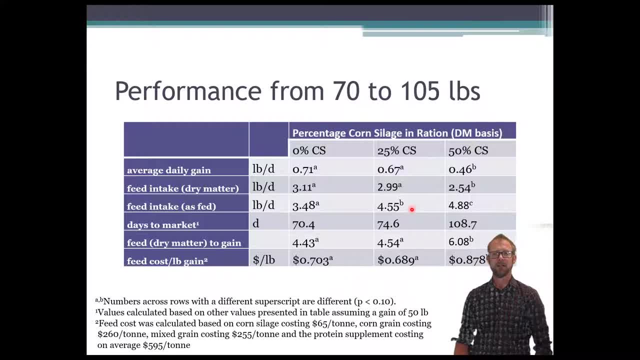 you have in there, the more feed there's going to be, because there's more water in it. corn silage is about 65% water, and so you can see that, yes, they did eat more feed. however, most that additional feed, of course, they ate was water. as a matter of fact, it all was water, simply because, if we look, 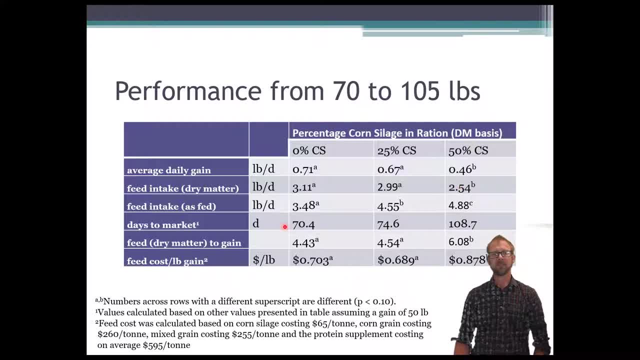 at the dry matter basis. you see it actually reduced this days to market number is not an actual number, it's a calculated number. I had made the assumption if the lambs gained 50 pounds, how much it would take them to do at these various growth rates, and it would take these guys about. 70 days about these guys about 75 days, probably very similar again because these two numbers were not significantly different. but then if we looked at the 50% corn silage would take about 109 days. you know that's 25-35 days longer. that's quite a bit longer time to go to market. and then the feed. 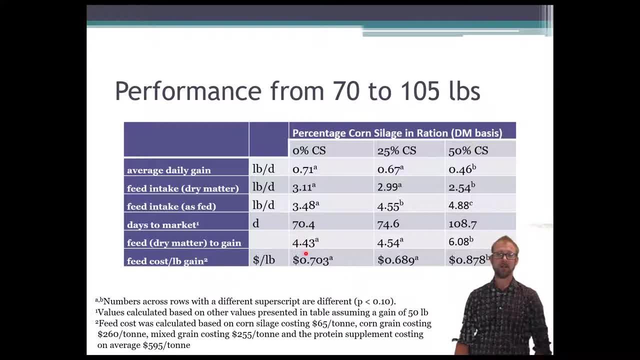 to gain ratio, okay, how much feed it takes to get a, how many pounds of feed to get a pound to gain, or how many kilograms of feed to get a kilogram of gain. you can see four point four, three, four point five, four, again not too high, but it's a pretty good number for that to be able to take a look at. on the other hand, I'm not saying that there's a specific number you can take a look at, but I think that you can take a look at the field and you can take a look at the number of days that you take. the number of days that you take. 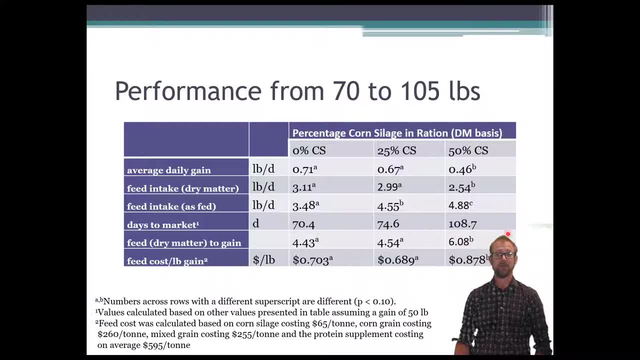 different, but this one here considerably higher feed to gain ratio, much less efficient. so even though that feed was so much cheaper, okay, the actual feed cost per pound of gain you can see was about 70 cents per pound, about 69 cents per pound for these guys but about 88 cents a pound for these fellows over. 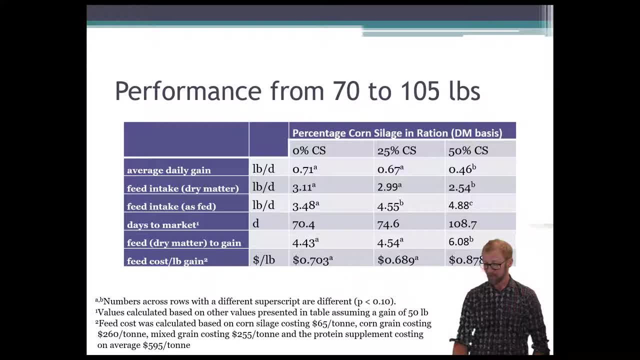 here. you could took it considerably more money to get them to go to market. if we can, we calculate out of this cost- ought to gain 50 pounds. we're talking about $35, $34 for this one and it would be 40- almost $44- for these fellows over here. 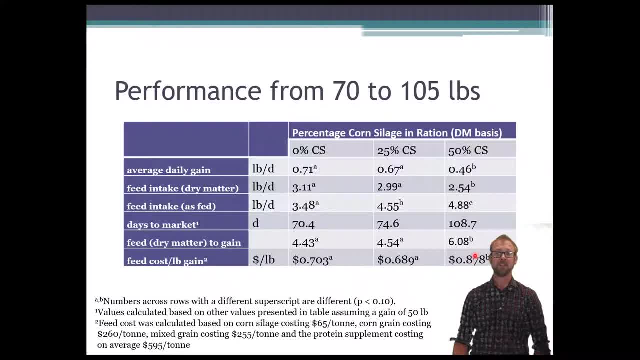 so considerably more expensive to get these guys up to market, even though the feeds cheaper, because that's lower growth rate and less efficient growth that we see here. it'll end up being not profitable to feed lambs at a 50% inclusion rate for corn silage- and, by the way, just to clarify, because that's a 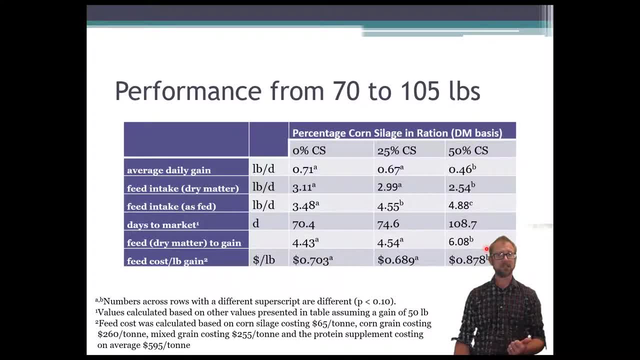 question I would get from time to time. this corn silage was processed and it was a low lignin corn, okay. so I have a question about corn silage and I would get from time to time. this corn silage was processed and it was a low lignin corn, okay, so I 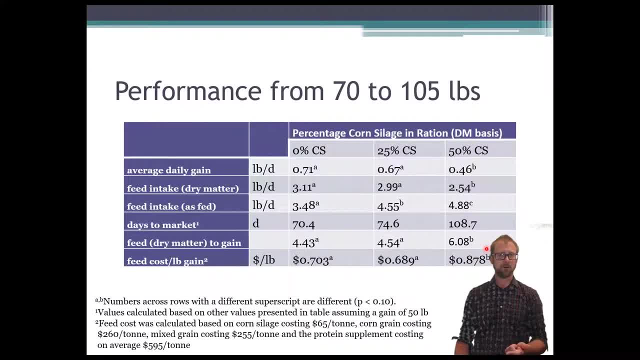 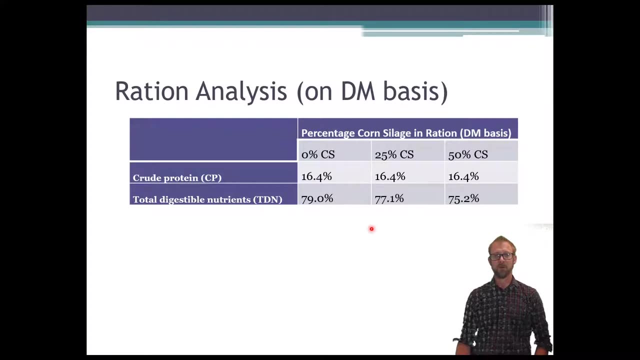 highly more digestible corn silage and it went through a kernel processor so it was broken into smaller pieces. so if any corn silage should have been successful with these lambs, this corn silage should have and in fact it was not. if we look at the diets we were able to, we targeted 16.4, we, I think we. 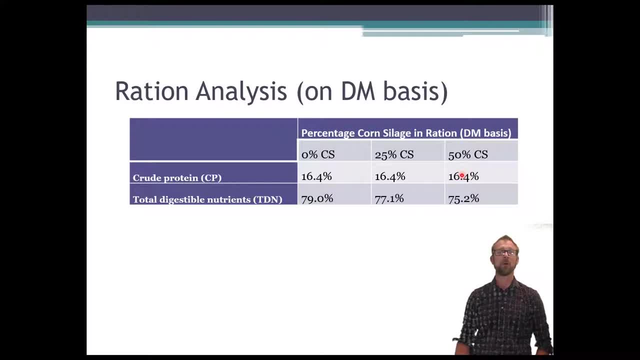 targeted 16%. we got 16.4% crude protein across the board for the diets and you can see that the total digestible nutrients amount of energy in the feed decreased and we were able to reduce the amount of energy that we were able to. 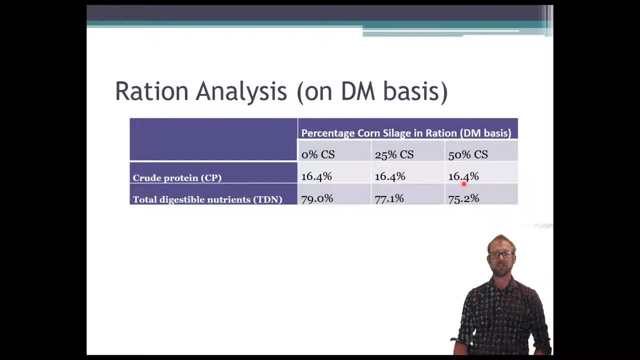 increase with more corn silage. again, that makes sense. what did we substitute for the corn silage, corn grain and mixed grain, which both have a higher energy levels. so the more we put in, the less energy there would be in those diets. I like to move on now to talk about some of the carcass measurements and some of 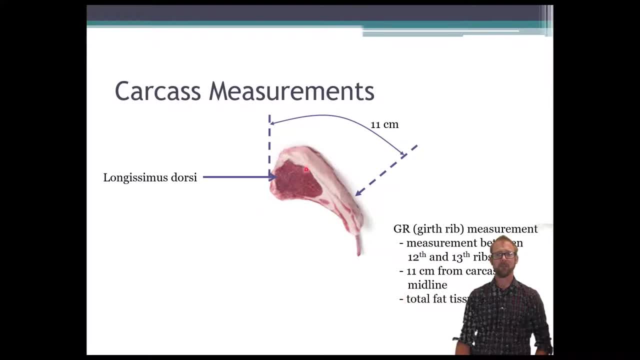 the things that we measured with that. before we get to the data, I just want to briefly explain what the GR measurement is. you may have heard of the GR measurement: girth rib measurement. it's a measurement between the 12th and 13th rib. so far, 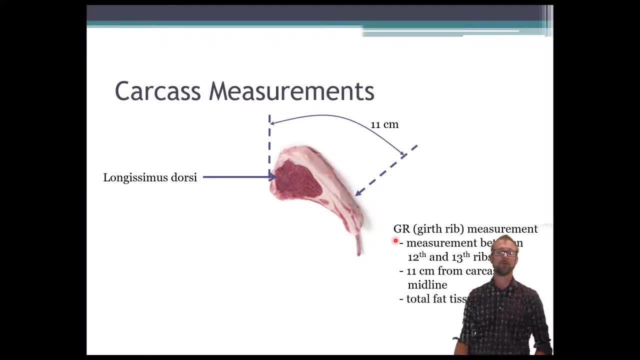 from the back to the 12th from the front, sorry, going to the back 12th, 13th ribs, and we measure 11 centimeters from the midline and the knife has a little kind of measuring scale on it that do, when you put the knife in, you can measure the. 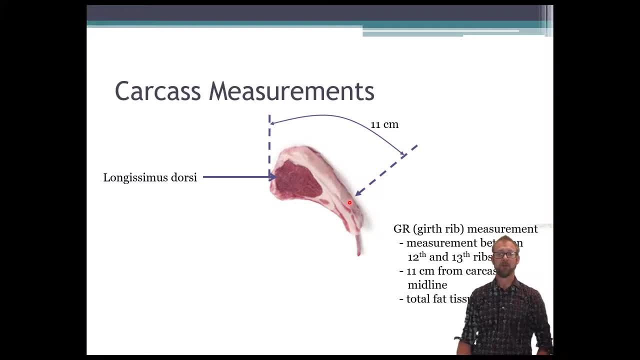 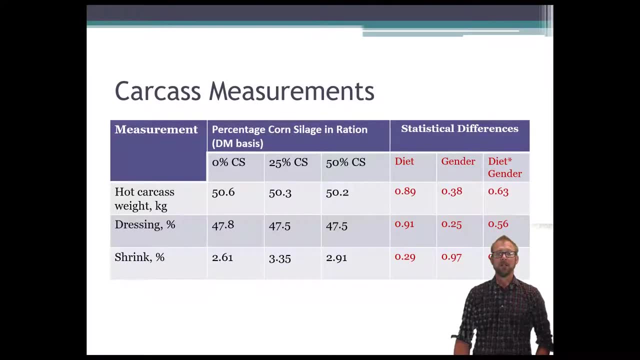 amount of fat tissue depth, and so that girth rib measurement will simply be a measurement of the fat at that level right there. so what did we get when we look? so do just explain this table a little bit. these are the statistical difference numbers over here. basically, the lower this number is, the more 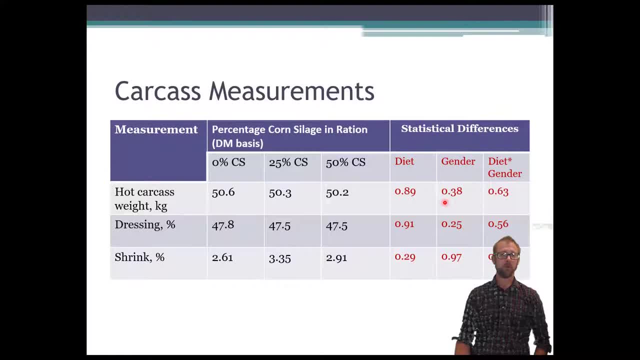 statistically significant it is. I declared significance at 0.1. that's not necessarily a magic number. some people go 0.05, and you can. you can choose where you declare your significance to be. certainly, though, if you see a number like 0.89 that's getting closer to one, the highest you could get would be. 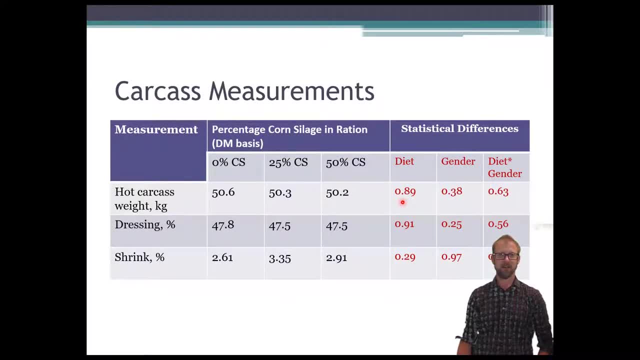 theoretically would be a one, and that would be completely no significant that, in fact, that what that would mean is that there was no treatment effect on the hot carcass weight. so the fact that this number is extremely high tells you that there was absolutely no impact of. 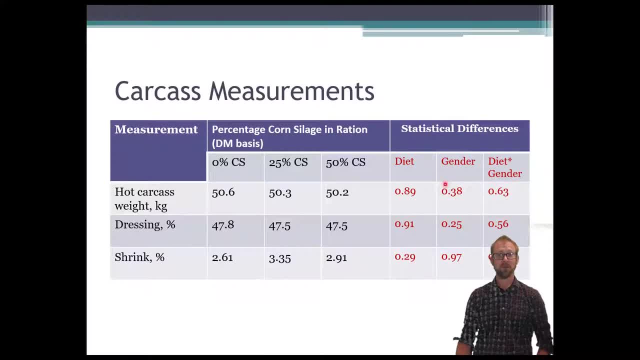 treatment on there. we also had either use or weathers and so we measured that and I might discuss it a little bit, but I'm not going to get into a whole lot of time talking about the, the gender differences, just because most of the differences that we were interested in was the corns level of corn silage in. 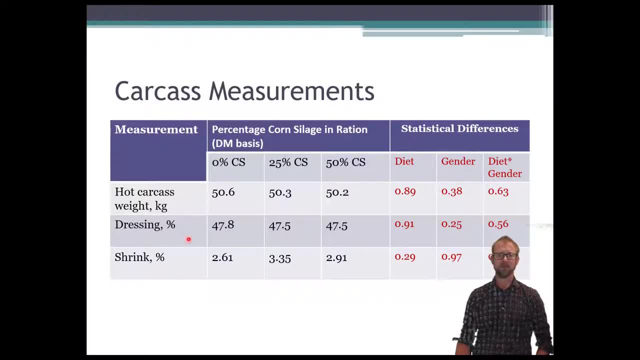 the diet dressing percentage, also again not different between the treatments. again, the trusting dressing percentage would be the amount of carcass there was after the animal has been cleaned, all the organs are out of it and the wool is off the shrink percent. that would be how much it shrunk in the day that, the day one that it cooled. and again there was. 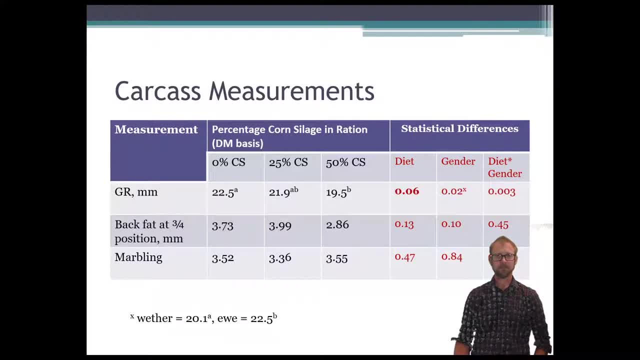 no significant difference due to diet. because of that, here you can see the number that that we're talking about here in terms of the GR and millimeters. the zero percent corn silage had a twenty two point five a millimeter a measurement. the twenty five percent was had as the letters a, B, which means it's. 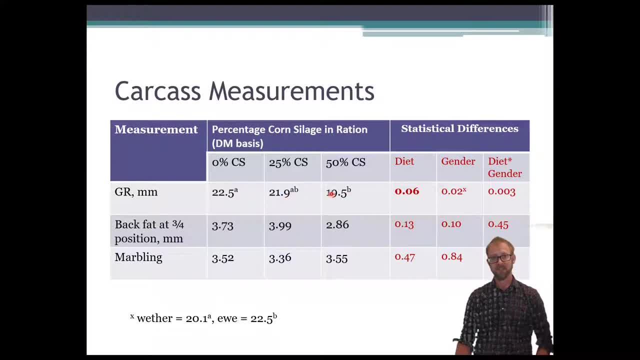 not different from this number or not different from this number, but in this case these two numbers are significantly different. the zero percent in the fifty percent corn silage numbers are different, and so you can see that there was less fat on the fifty percent corn silage lambs and this was significant. 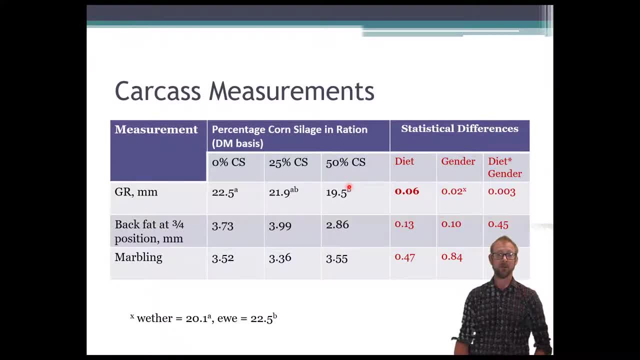 there was a significant difference there. that tells me again that probably there don't they just sell. it says at that point there was less fat on them. if we looked at the back fat, at another measurement of back fat, it was not significant. this case you could see which. 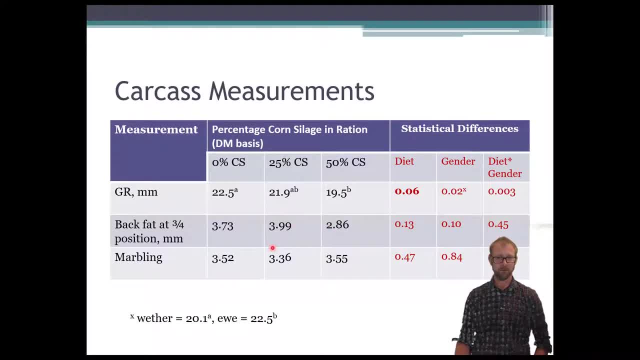 was kind of close and again, numerically you can see kind of the same trend as we saw for here. this is interesting because another way we can talk about fat is the marbling, that's the fat that's interspersed within the meat and that's 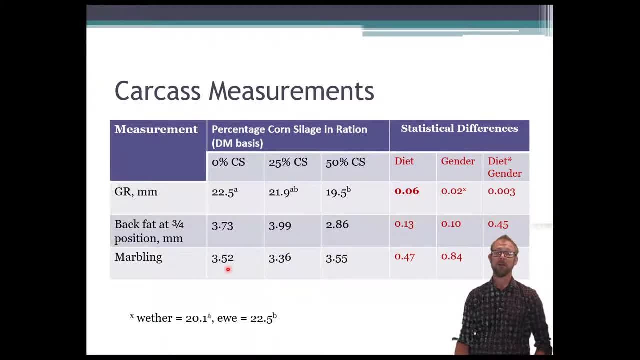 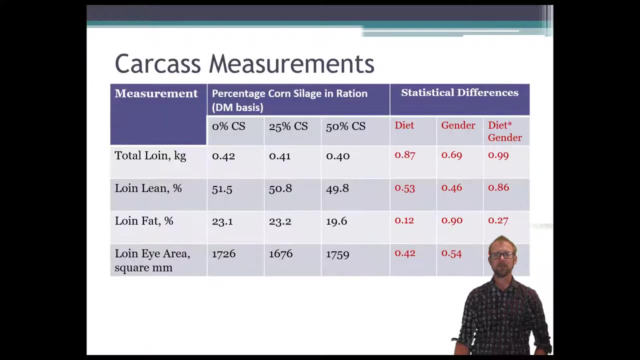 usually we think about that in terms of flavor and tenderness and so forth, and so the higher number in this case would be a good thing, and we saw actually that the treatment did not have an impact on marbling. this would be, so it looks like maybe the difference in fat levels was mostly a back fat level issue. if we look 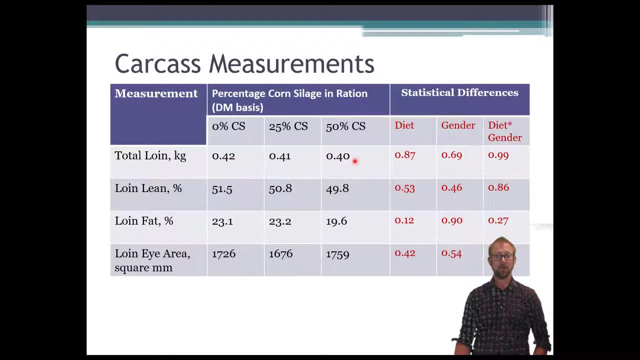 at the loin: okay, again there's no difference in terms of the total weight of the loin, no difference in the loin lean a loin fat, again not significantly different, but again this number kind of matches up with what we saw on the previous screen. and then the line eye area: again there was no difference. 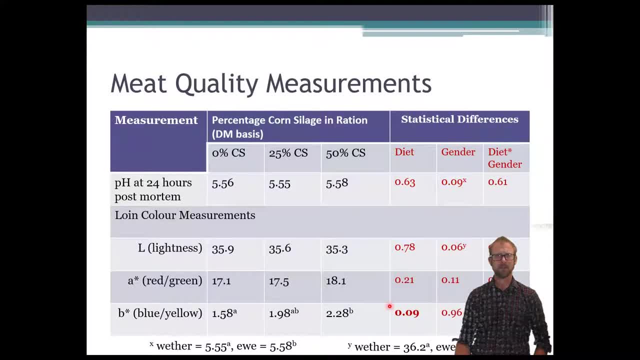 across the treatments for this one either some other meat quality measurements. we took the. if you look here, you can see the pH at 24 hours. again, there's no difference due to the diet. there was a small difference due to gender and I had those numbers down here: 5.55 versus 5.58 I. I doubt that that is a biologically significant. 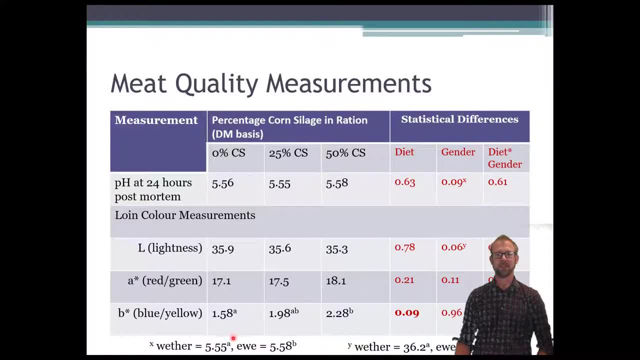 even though it might be statistically significant difference, I I would be surprised that that would be a biologically significant number. the other thing we did is we measured the color, and so the camera that can measure color and lightness, and again we found no difference. due to treatment, due. 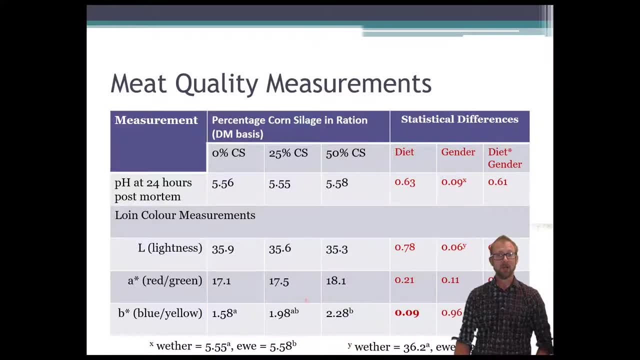 to the lightness, the red green colors. we saw no difference. we did see a difference between the- again, the zero percent and the fifty percent on the blue yellows: um number difference. uh, we saw a difference there. I talked to the meat scientist about this and he 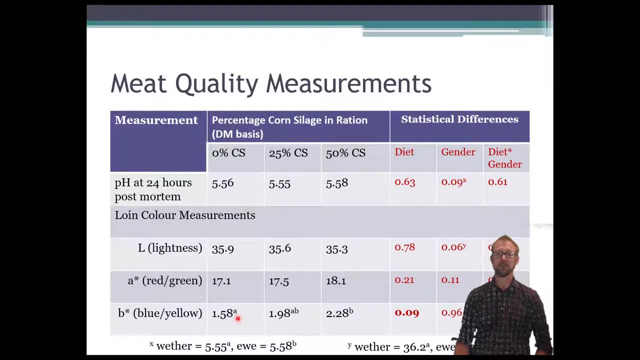 said again, this difference though there it may be, statistical, mathematically significant difference, is probably not a biologically significant difference. no human would be able to detect that difference between those two colors. again, there were some gender differences and I'm not going to go into a lot of detail to talk about talk about those at this point in time. 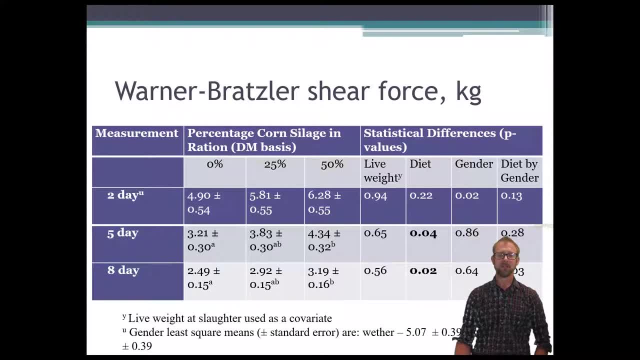 another thing that, uh, we were able to measure is a shear force, and let me just kind of explain how this piece of equipment works, and if you're a meat scientist you might cringe at my explanation of it. but basically you, you cut a core of meat, a round core of meat, and you set it in this machine and 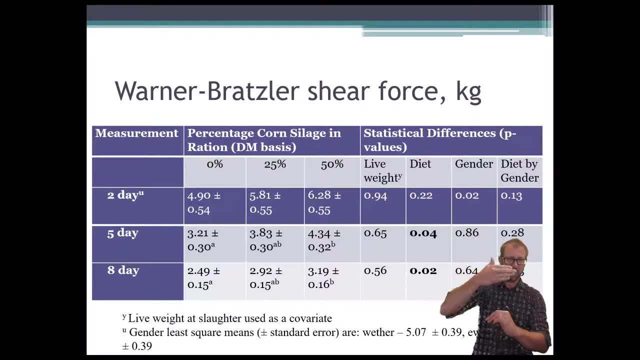 there's a knife that comes down, and the knife will come down at a set speed. coming down and how much pressure it takes to cut that meat will then, uh, be the shear force. the more tender the meat is, the less force it takes to to cut it. so it's kind of a measurement of the tenderness of 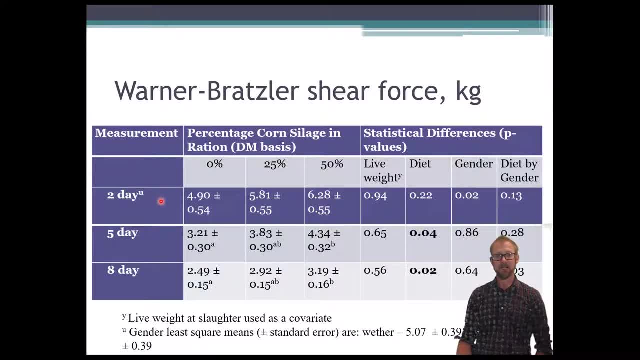 that piece of meat. now we have that we. that was done at two days, at five days and at eight days, and so here you can see the averages, with the standard uh error with it, of each of the numbers as well. as far as the statistics went on this one, we use live weight as what we call a covariate that 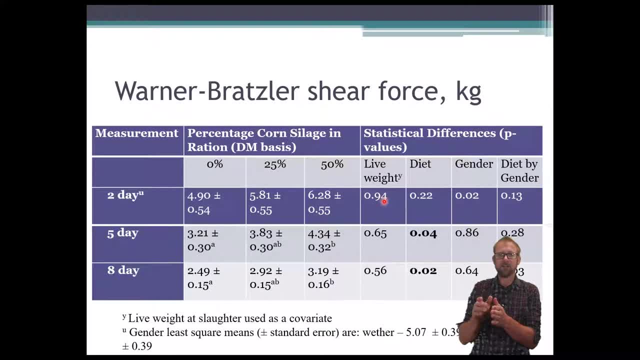 means we said whatever the weight was when the animal died is going to be, they're going to be corrected for that weight. because the 50 corn silage ones were a little bit lighter in general when they went for slaughter. we want to be able to correct for that, although you can see that that 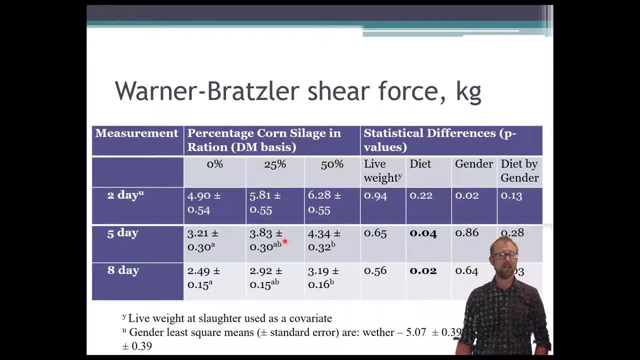 impact didn't actually impact across because none of these were actually affected by the weight of the meat that were significant did not actually impact the um, the tenderness of the meat at the for the treatments and across the different days. there you can see again a little bit of a difference here. 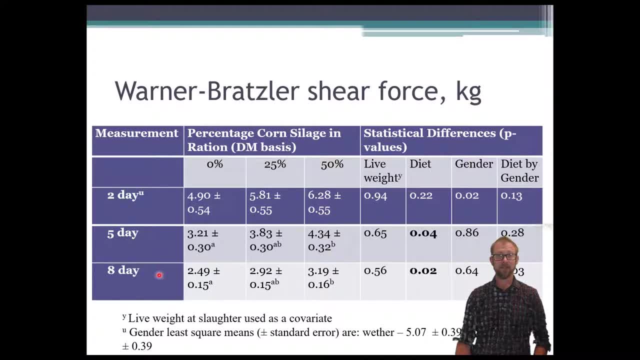 for a gender on day two, but as we move up here to day five and day eight, there was a difference due to diet and again you can see that these ones took a little bit more force. the 4.34 versus 3.21, um, it took more force. there was no difference between these, but you can see. again there's a 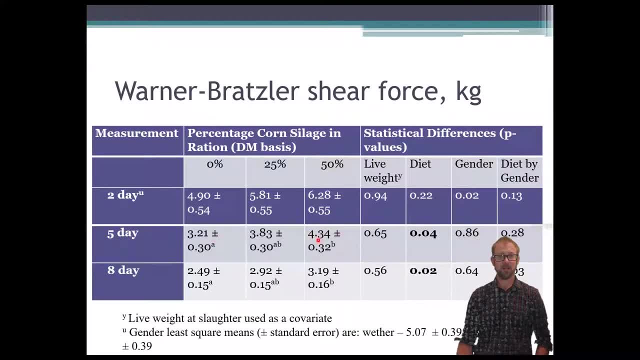 trend. uh, I would say that you can see kind of a linear uh a line there and same with the. the eight days it got tougher and again there was a significant difference between the, the lambs at um 50 corn silage versus the lambs at eight that were at 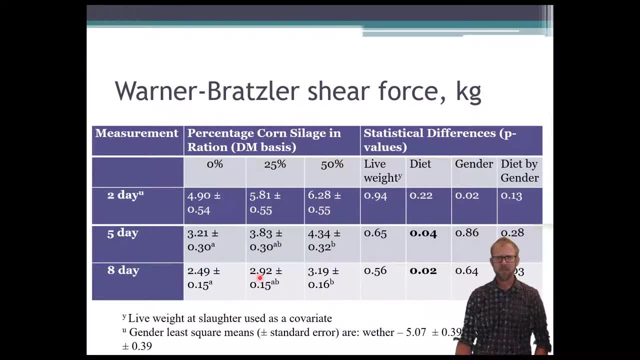 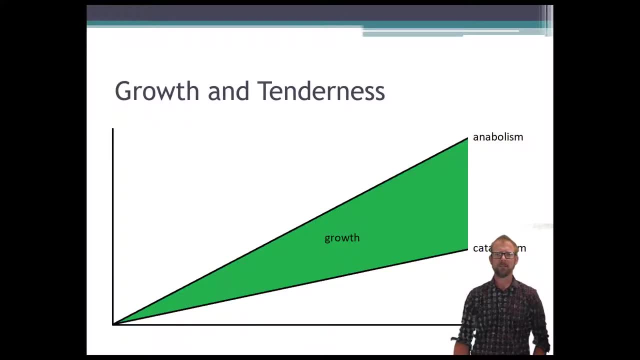 uh, zero percent corn silage at the tenderness at eight days. now I I made this next slide to kind of explain that and again it's. it is a generalization of how it works, but I think it's a. I think it's a fairly good explanation of it. anytime you have growth going on in an animal, you have. 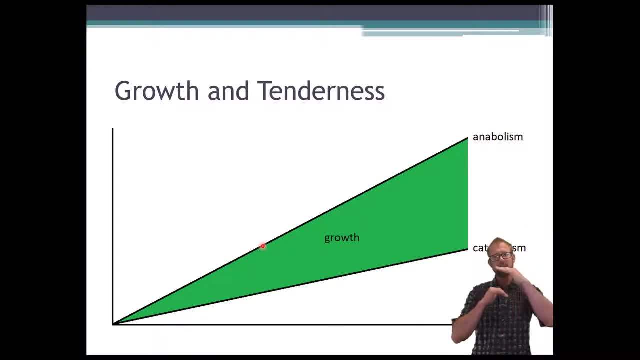 anabolism. anabolism is the, the actual growth, but at the same time you always have catabolism going on as well, and so the catabolism, uh, and and any and. as anabolism goes higher and higher and higher, so does catabolism. it goes up as well. just it doesn't go up as fast, and therefore the green 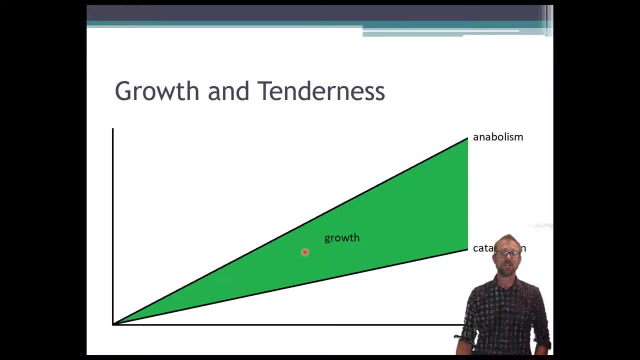 part you can see the growth of the animal. it gets larger and larger. so the generally, in general, the faster an animal is growing, okay, the more and of course the more anabolism is going to have, but also the more catabolism that's going to be going on. 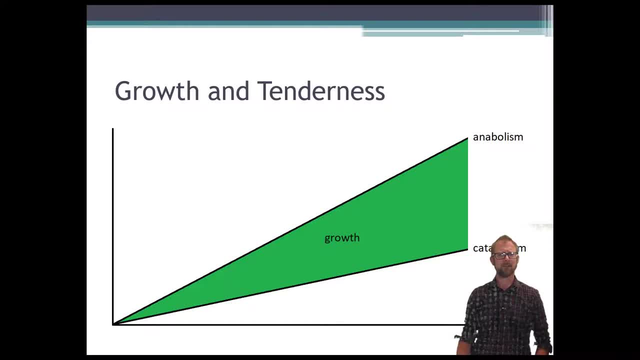 um, this has become important when we and when we go back and look at that, uh, that previous slide, and we see that the ones that were growing higher tended to be faster, tended to be more tender. well, when I slaughter that animal, okay, when I slaughter the animal, and let's say it's at this point, right. 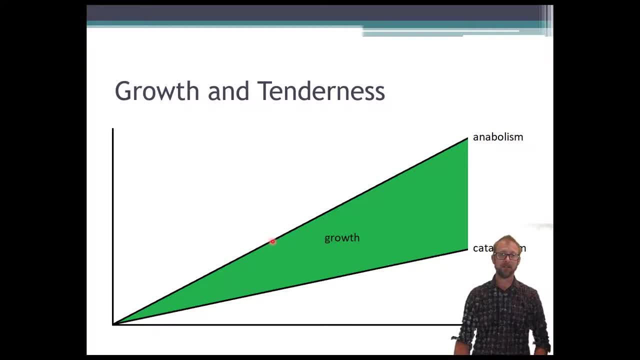 here. I have one animal that's right here and I have one animal that's over here. okay, down here. at this point, once I slaughter them, the anabolism stops. okay, they don't grow anymore. however, the catabolism in lambs can continue for about a week. okay, they'll continue, at least at a significant. 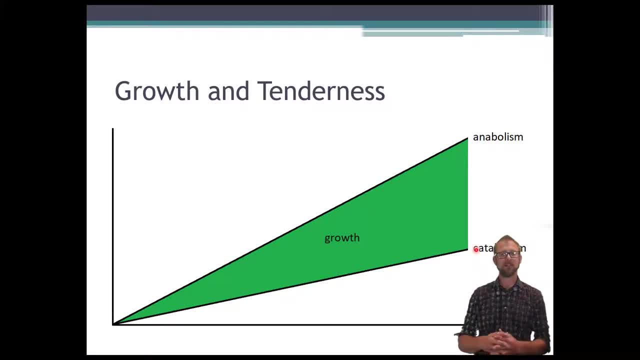 rate and so that in the second catabolism that tenderizes that meat, it breaks down some of those tougher proteins and proteins that are going to be harder to chew and so forth. and so the faster that animal is growing, the faster the catabolism, which means after a week you're going to have a. 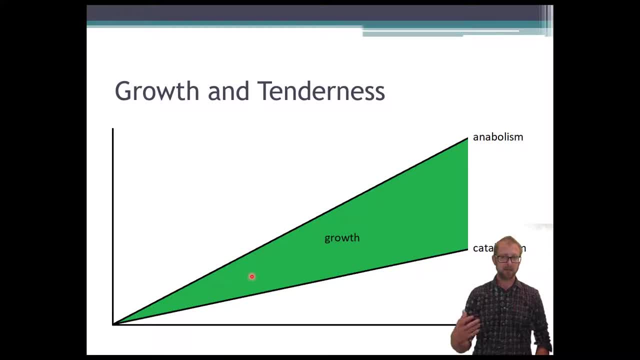 higher amount of those proteins broken down and the animal is going to be more tender. this is one of the reasons why, too, if you're going to call an old you, if you can put her to feed for the last maybe week or two before she's slaughtered, before you send her off, she will gain some she can gain. 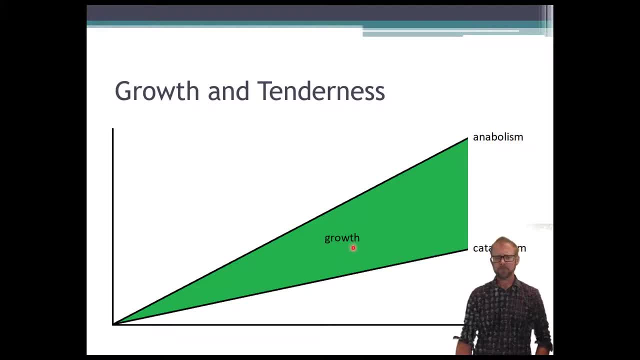 less fat, you can actually make her a little bit more tender. so in general, the quicker they're growing, the more tender they're going to be, and we saw that in in this particular trial. another question people might be wondering about is: what impact does the corn silage have on feed? 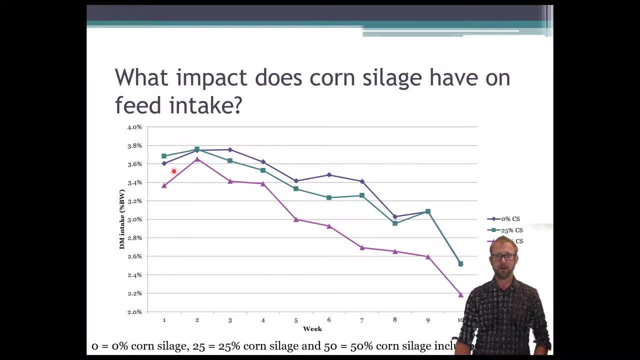 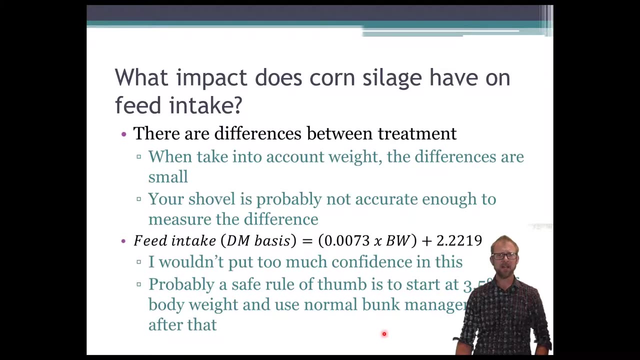 intake. so we did. I just plotted the numbers across here and this is a feed intake by a week and again you can see feed intake was relatively constant for the 0-25 and it was lower for the the 25. to do is: I tried to develop some equations to build to predict this, and when I did that once I 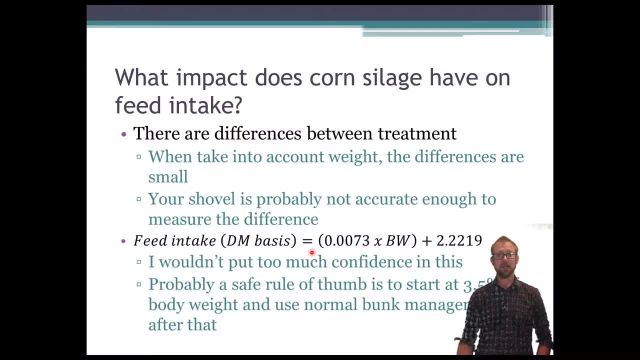 take into account the actual weight of the animal, can keep it in mind that that in that previous slide those ones out, the growth, the feed intake was slower for those corn silage ones that corresponded with their weight being also later, if we would shift it over so that they're at the same. 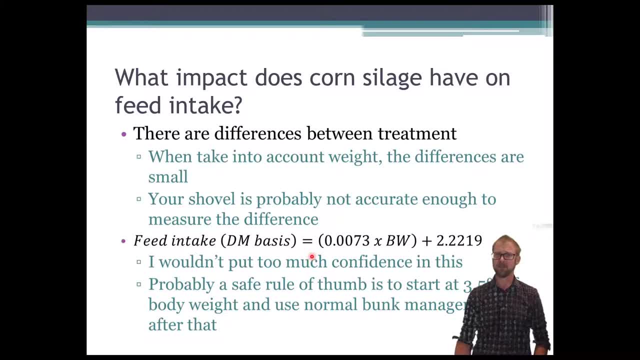 weights. there was very little differences between the different treatments in terms of their ability to feed intake. it's so much so that I really don't think that it's probably worth worrying about. I say, oh, the level is probably not accurate enough to measure the difference that you might see, so I did. 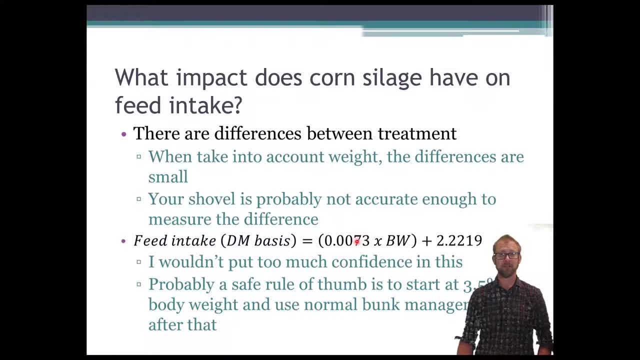 develop this equation here to predict feed dry matter intake based on the feed body weight of the animal, I wouldn't put a whole lot of confidence. I mean, the equation works. I think it's fine. however, I think this is a safe rule of thumb if you start at three and a half percent of body weight. 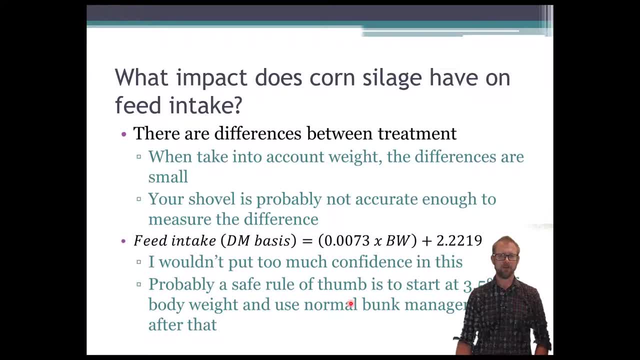 and then just use bunk Management practices after that. I think you're going to be doing well. and so, again, you weigh the total number of lambs. you got 100 lambs in a pen, all their weights together. take three and percent of that and that would be a good place to start in terms of feed intake for those lambs. 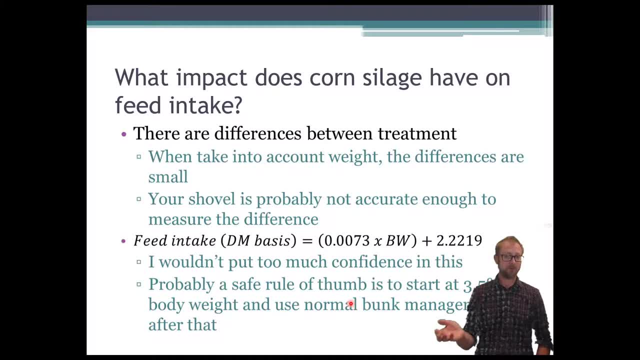 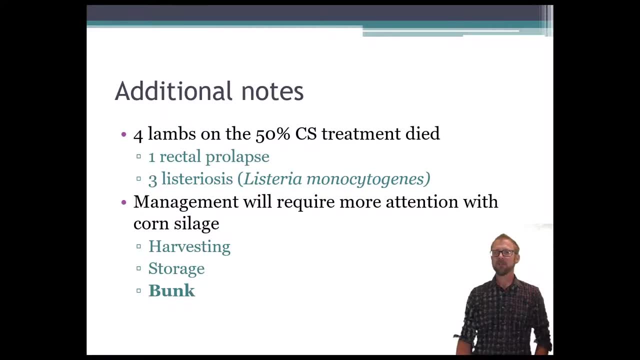 After that you can decide whether you want to feed, for example, 5% refusals, or if you want it to be slick bunk. whatever the case is now, you can manage that. Some additional notes that I think are very important. We had four lambs on that 50% corn silage treatment that died. 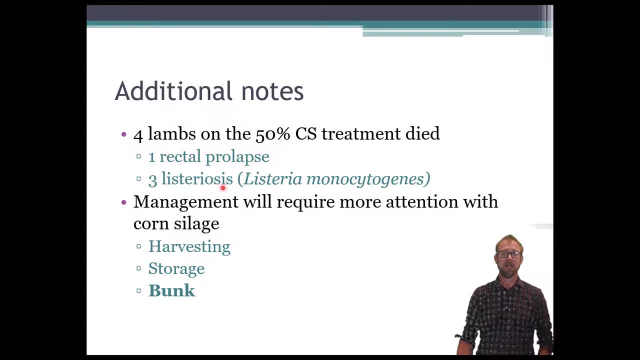 One had a rectal prolapse, Three of them died of listeriosis And to me, this is this basically. in my opinion, this is a game changer for using corn silage. So listeria is a bacteria that's very. 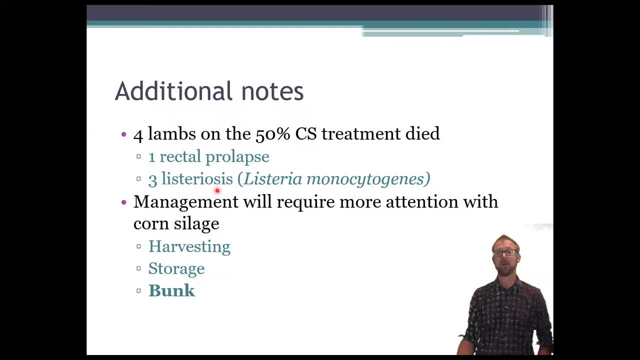 common in our soils and so forth, and it thrives in warm environments and also thrives in moist environments and in oxygen-rich environments. So when we put our feed in our silages, in our silos, we try to get rid of the. there's of course going to be moisture and, depending on the time of year, 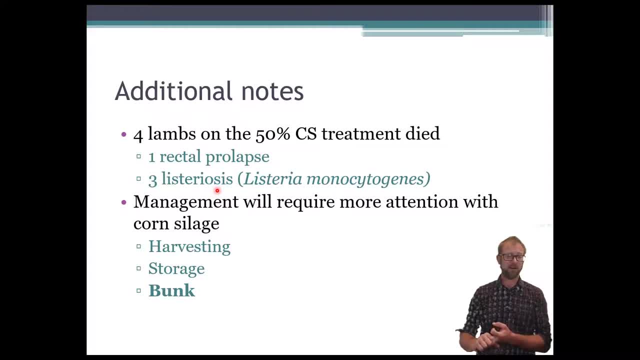 there could be heat in there, and so we have to do a really good job of getting the oxygen out of there, And that's why we pack bunk silos and that's why we try to fill silos as quickly as possible, And that's why we have to remove so much feed every day, because the oxygen will start. 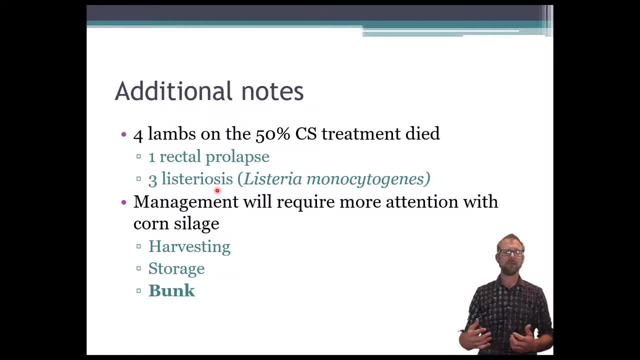 allowing this bacteria to take over. So it's often a bacteria we think about when we're talking about feed spoilage And basically the bacteria gets into the brain of the animals and it causes circling disease, where you see them circling, and fairly quickly it turns into. them laying down and they can't get back up and they'll paddle and it will kill them. If you catch it early enough, you can't treat it with antibiotics, but you have to be right on it to catch it And your time. the time frame is relatively small. 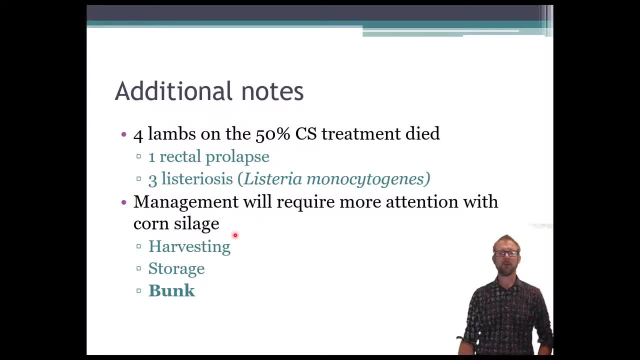 So if you're going to be feeding a corn silage diet, you're going to have to spend more effort and more thought on your management for that Harvesting in the first place, to make sure you don't get soil contamination into your feed Storage again making sure you get as much. 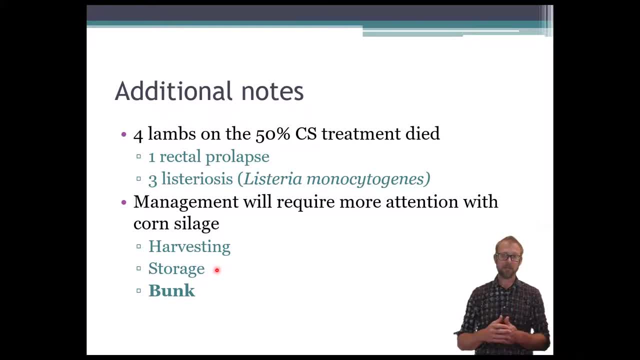 oxygen out as possible. Make sure you remove the correct amount of feed, For example, bunk silage- you should be removing six inches a day to stay ahead of that spoilage. And then bunk management. Your bunks have to be cleaned out. I would say at least six inches a day, And then 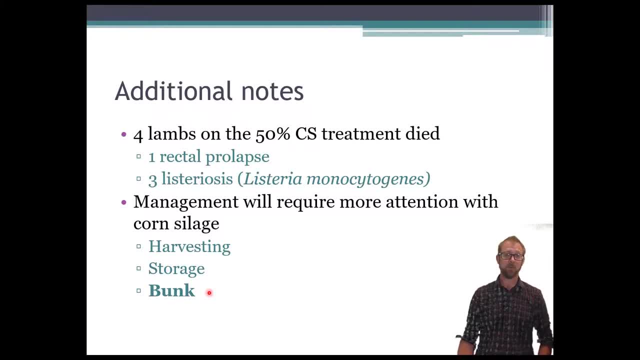 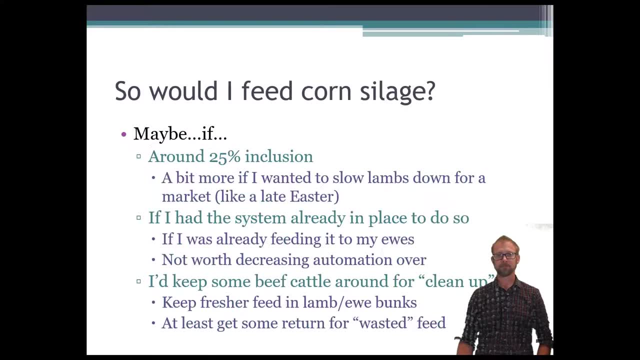 at least once a day in cold weather and twice a day in warmer weather. they have to be completely cleaned out because that feed spoilage will increase the risk of listeriosis. So the question comes is: would I feed corn silage? Probably not, However, I'm going to say maybe. 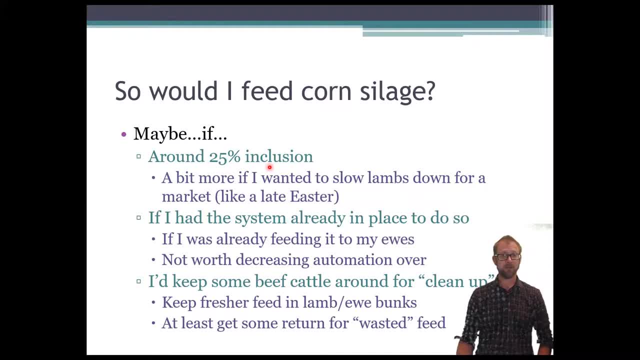 Maybe, if I maybe- around 25% inclusion. we saw no difference between the 0% and the 25%, And so I could have, for example, if I wanted to slow lambs down the next slide. I'm going to talk about this. 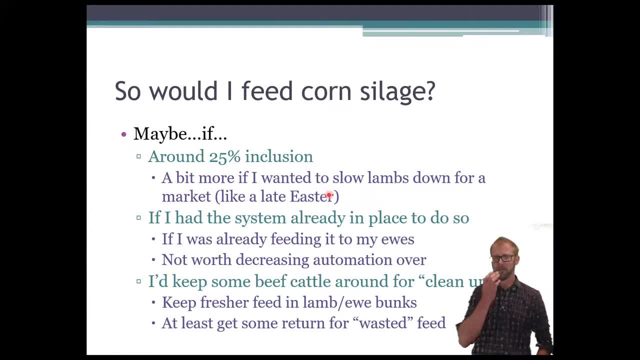 a little bit. I wanted to slow lambs down, basically background them for a little bit in order to be able to hit a later market. Okay, The other thing I would need to have is I'd already have to have a system in place to do so. I'm not going to be buying silos or ag bags or a mixing cart or anything. 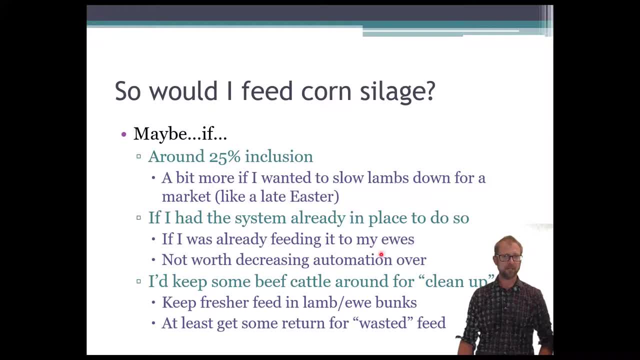 like that for feeding lambs. However, if I'm already feeding my ewes like that, then maybe I would decide to feed a little bit of corn silage them as well. I really don't think, though, it's worth decreasing automation over. It's much easier to automate systems when you're feeding. 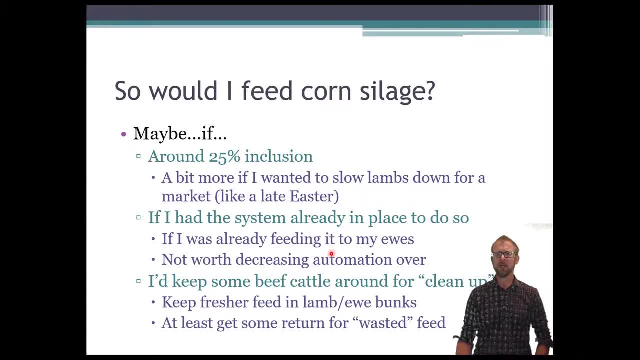 grain than it is to feed with corn silage or forages, or wet forages- I should say silages. And so I. this is probably one of the big reasons why I wouldn't do it labor. If I was going to do it, I'd like to keep some beef cattle around for cleanup. Beef cattle can get listeriosis as well. 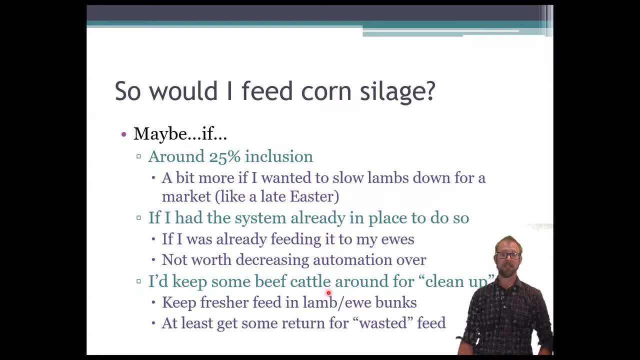 but they're much less susceptible to it, And so if I was going to clean out my bunk twice a day, I could then throw the refusals to them and they could clean that up, And at least I don't waste as much feed, Maybe instead of feeding for 5%. 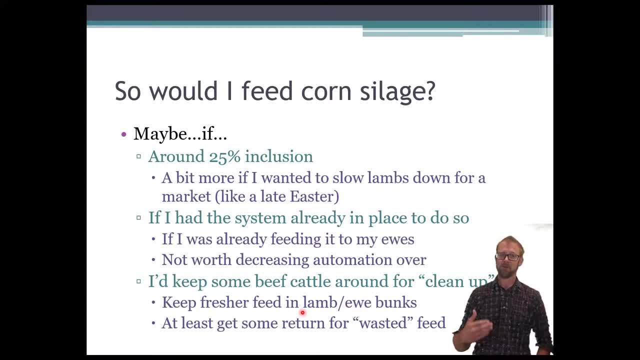 refusals. I could clean that up and at least I don't waste as much feed. Maybe instead of feeding for 5% refusals, I could clean that up and at least I don't waste as much feed. Maybe instead and I feed for 10% refusals, and that will help those lambs be able to have fresh, clean feed in. 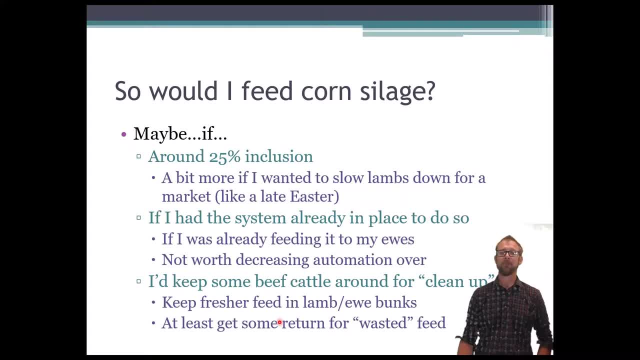 front of them for longer and more, for a longer period of time, But it'll, they'll flip and then I can feed that to the, to the, those beef animals, so that it doesn't get wasted. Let me show you just some calculations where an example where it might be beneficial to do this. Let's say I: brought in some lambs. Let's say we have a late, a late Easter, the particular year I looked at, an actual year when I was doing this calculation and Easter was shortly after April 18 that year, so fairly late, late Easter. And let's say I bought in. 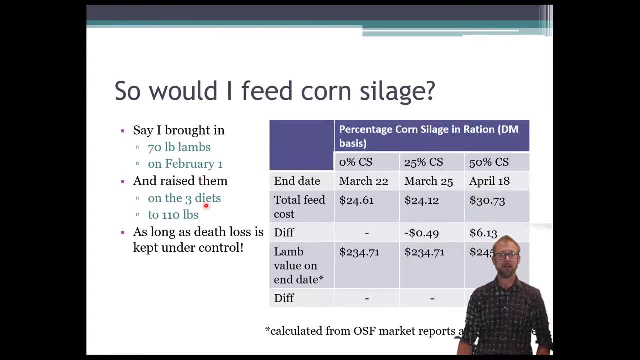 some 70 pound lambs on February 1st and I could and I raised them on the three diets to 110 pounds. If I was going to do that, these guys would be ready to go to market at 0% corn silage on March. 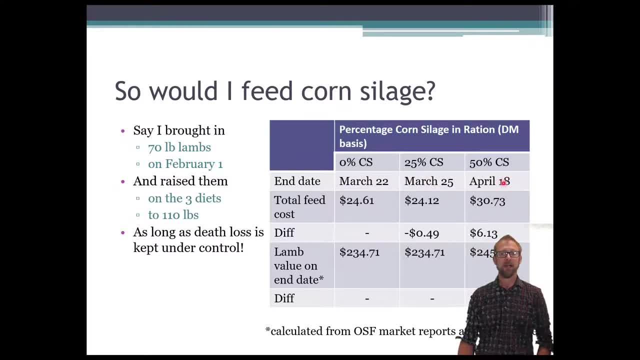 22.. These guys would be a couple days later, March 25th, And these guys would be quite a bit later at April 18.. If I look at my feed costs, based on how we did the calculation earlier, $24, $24.. 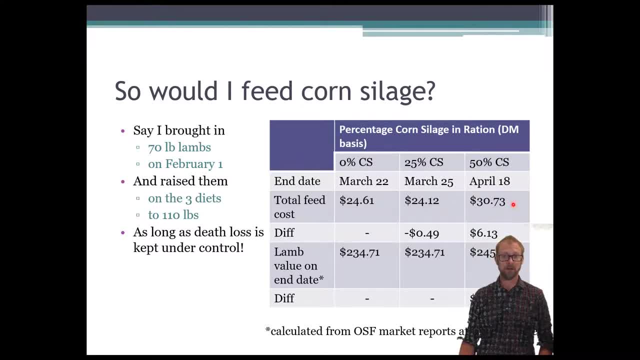 These guys are going to be almost $31 for feed costs, So I'm going to be able to feed them at a considerably higher cost than these ones over here: $6,, a little more than $6 more expensive And then. but then if we look at the actual value of that lamb at the end date, these guys would 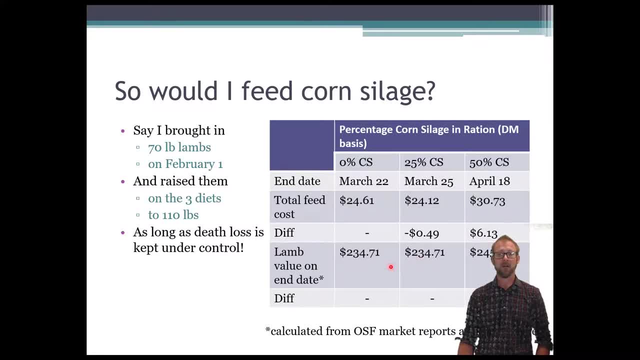 have gone to market before the Easter market was really starting to heat up. It was, it was coming up a little bit, but it hadn't really heated up yet, And so therefore they made about $10 less than if I was able to sell them on that later date of April 18th- And yes, I 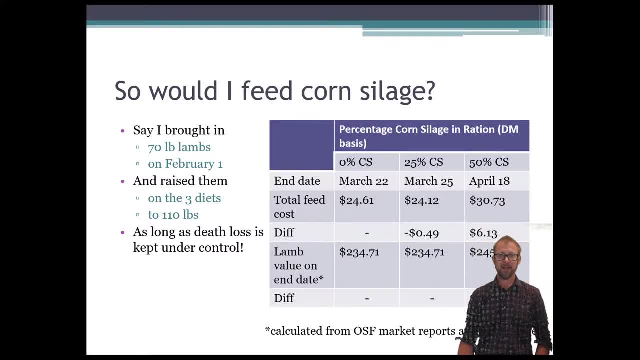 I'm losing $6 in terms of feed. here, However, I'm gaining $10.. I'm still about $4 ahead by by slowing them down. So in that situation, again, I think that if you want to slow animals down,